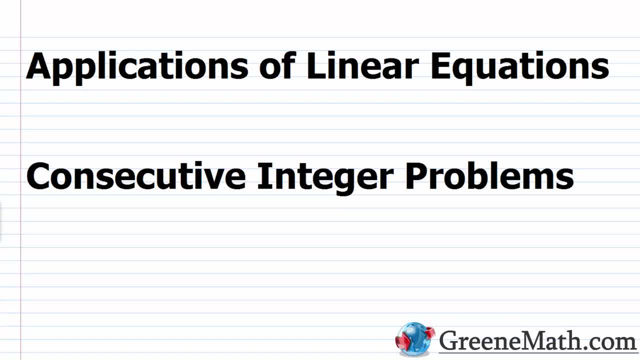 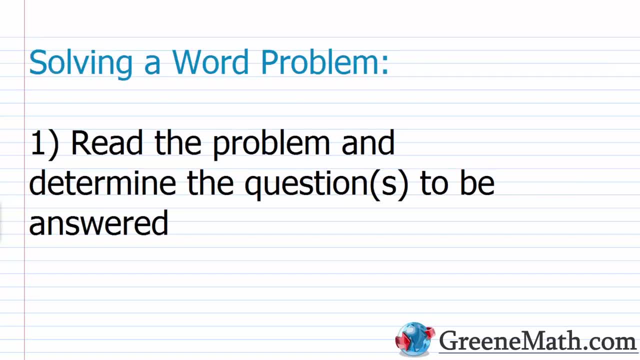 In this lesson we want to review applications of linear equations and talk about consecutive integer problems. All right, so once again, when we have an application problem that involves setting up and solving a linear equation in one variable, we have a little six-step procedure. we 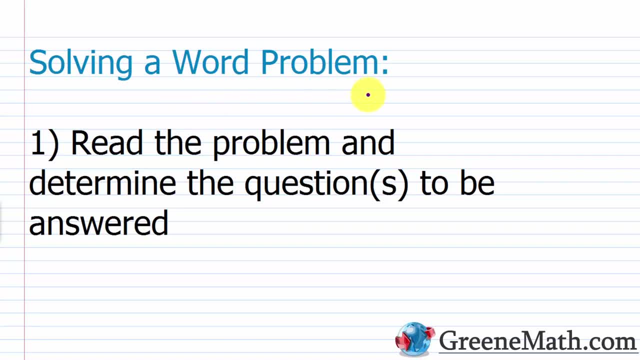 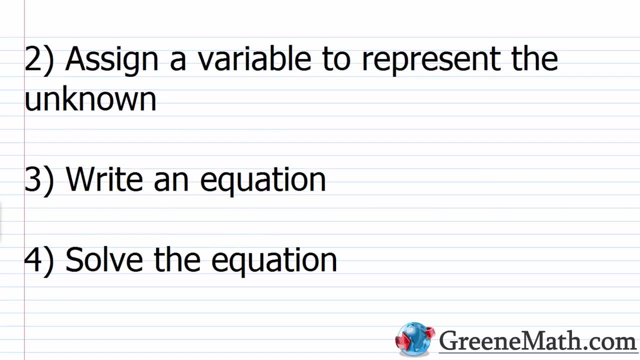 can use. So for solving a word problem, the first thing we want to do is read the problem and determine the question or get questions to be answered. Then we want to assign a variable to represent the unknown, And then in these type of problems we can always express any other unknowns. 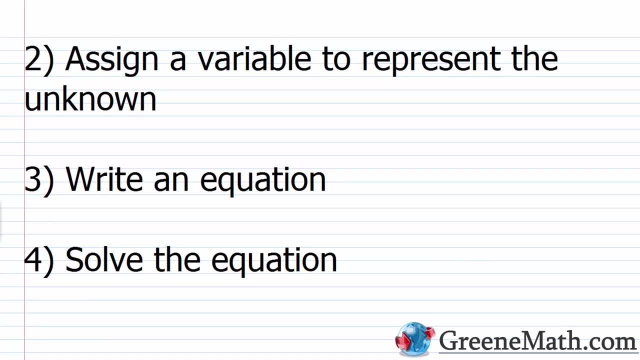 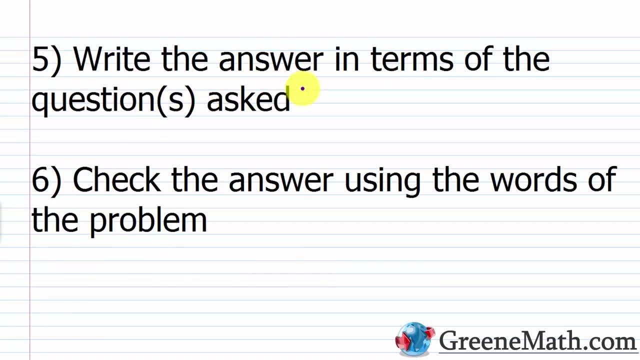 in terms of this original variable. Then we're going to write an equation. This will be based on the situation given. We're going to solve the equation, Then we're going to write the answer in terms of the question or again the questions being asked. Then, lastly, we're going to check. 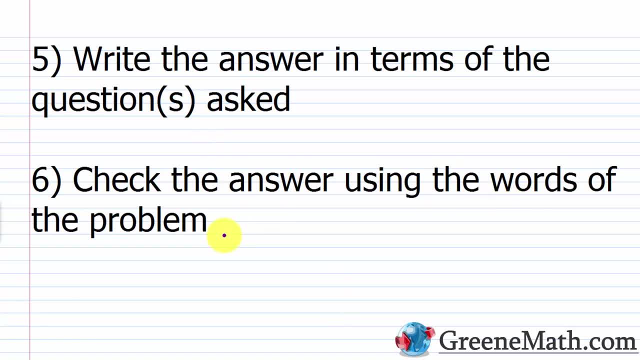 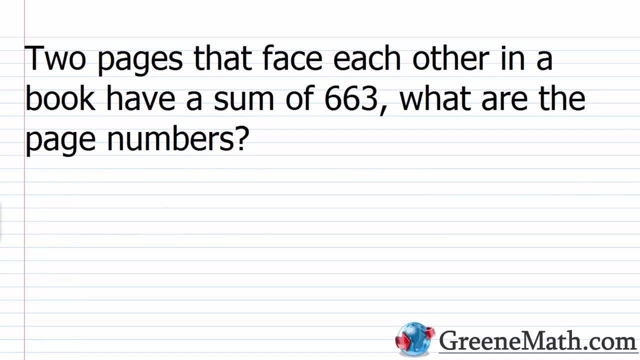 the answer using the words of the problem. We always want to make sure that our answer is reasonable. All right, so let's just jump in and look at a problem. These problems are very easy to understand and solve, so you really shouldn't have too much of. 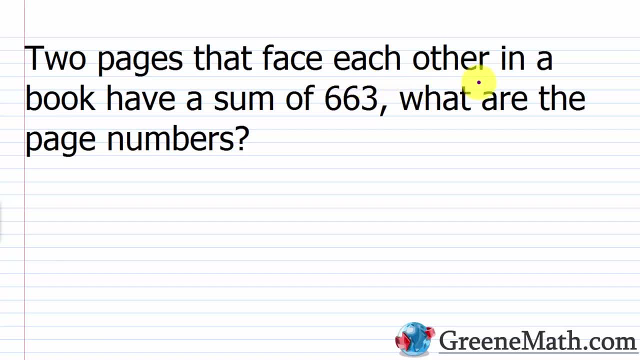 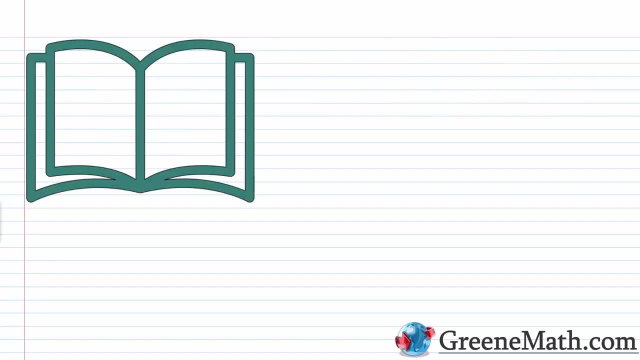 an issue with them. So two pages that face each other in a book have a sum of 663.. What are the page numbers? So, to get an idea of what's going on here, if you think about a book and you think about two pages that face each other, you could say this page is one and this page is two, right? 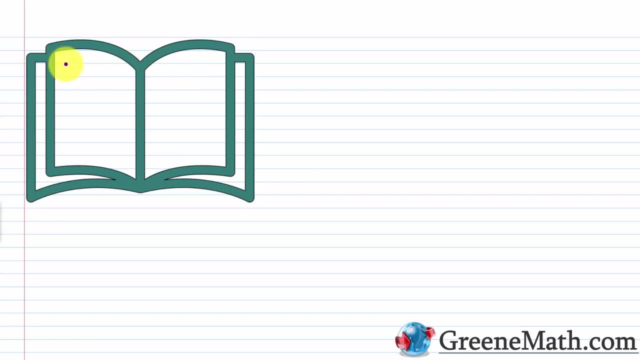 They're going to differ by one. Or you could say that this page is, let's say, 500 and this page is 505. So you could say that this page is 500 and this page is 505. So you could say that this page. 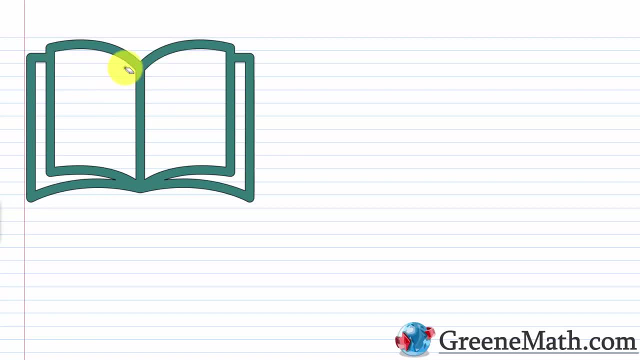 101, you know something like that. So we know that the smaller page could be represented with a variable like x. So let's let x be equal to the smaller page. Okay, let me make that better, Okay. so then, what can we say about the larger page? Well, it's just one more right In the 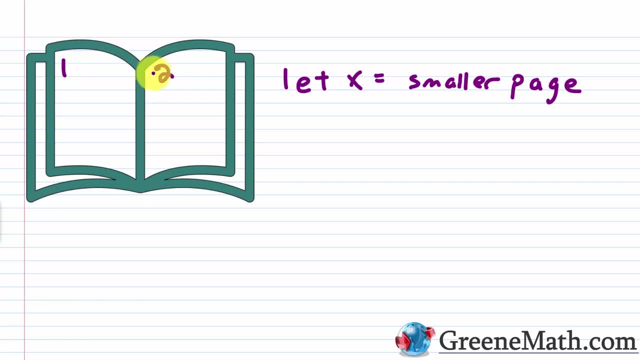 instance, where we had one and two, one was the smaller, two was the larger. it's just a difference of one, Okay. So what I can say is that we could say then: x plus one is the larger. okay, the larger page. Okay. So what we're told is that the sum of the pages is 663.. So it's very easy to solve this. 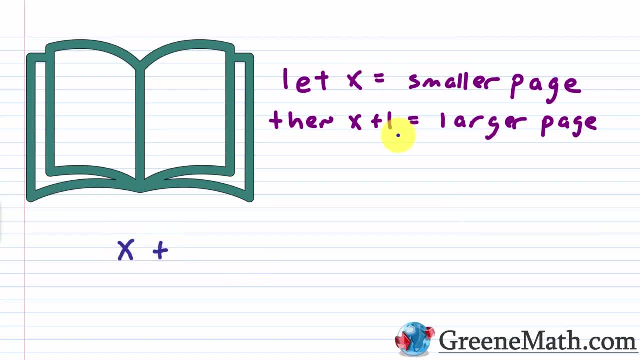 I just take my smaller page, which is x, and I add it to my larger page, which is x plus one, And this equals 663.. Okay, So all I got to do now is just solve my equation Very, very easy. So if I just remove the 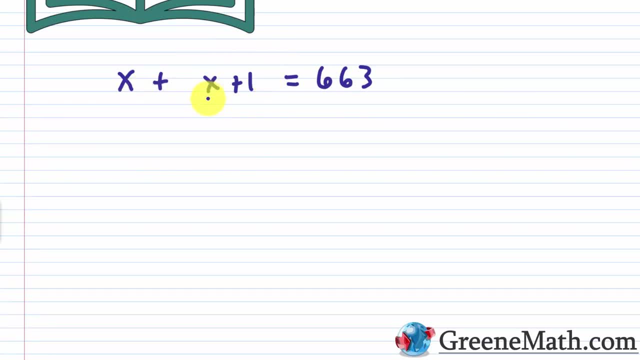 parentheses here, because I don't really need them. x plus x is 2x, And then plus one equals 663.. Let's go ahead and subtract one away from each side of the equation. We know this will cancel and you'll have: 2x is equal to 662.. Let's now divide both sides of the equation by two. 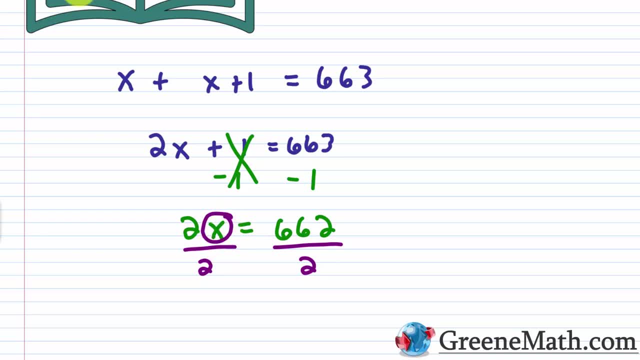 so that we can isolate the variable x. So we know that this will cancel with, and I'm going to end up with: x is equal to 662, divided by two is 331.. Okay, So again, when you work with a word problem, you can't just say x equals 331 and turn in the test. right, You got. 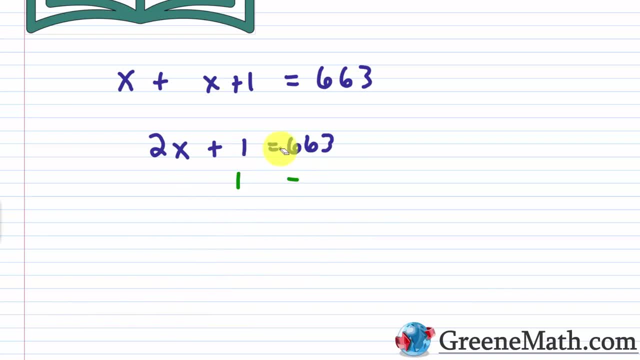 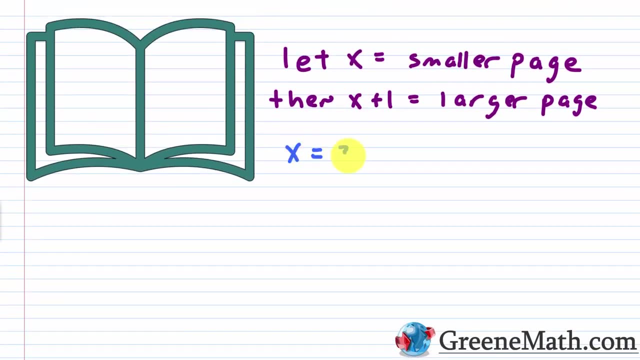 to make sense of it. So let's erase all this. I'll show you in our little picture what's going on. All right, So if we come back up here again, we said x was equal to 331.. This is the smaller page. 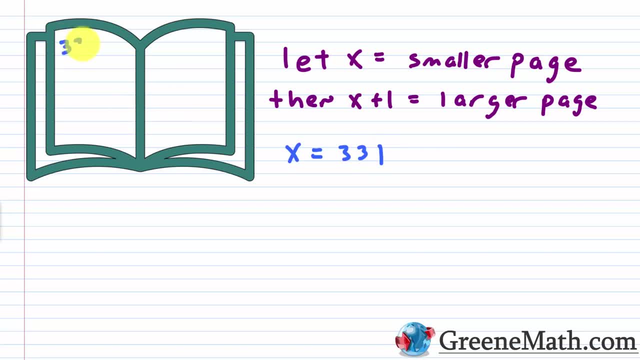 So in our book we could say: this page here is 331.. And then the next page, the page that faces that one, is going to be 332.. Okay, And you could check. that Is the smaller page 331?. Well, if the larger. 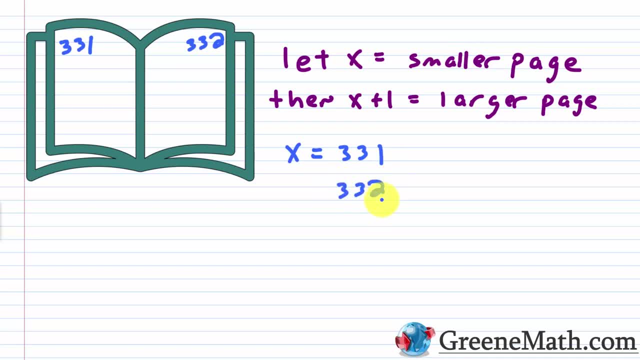 page is 332,. if you sum those two amounts together you do get 663.. Okay, So everything is consistent with what we're told in the problem. So let's go back up Again. what are the page numbers? So to answer that question: 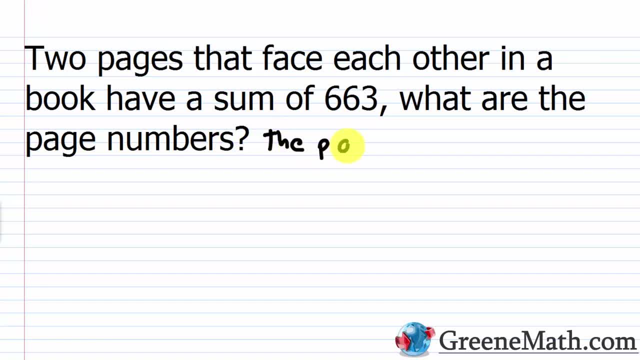 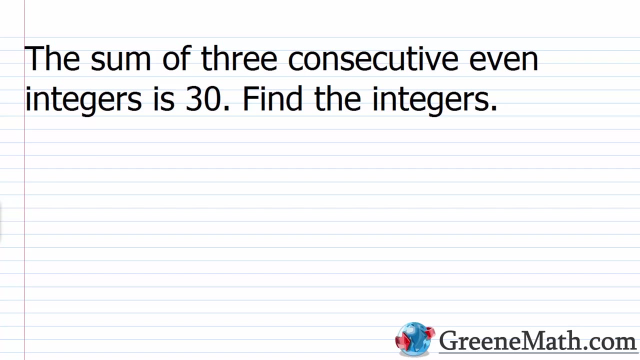 we could say the page numbers are again 331 and 332.. Okay, nice and simple. All right, let's take a look at another one. So the sum of three consecutive, even integers is 30.. Find the integers. So in this particular case, you've got to understand what it. 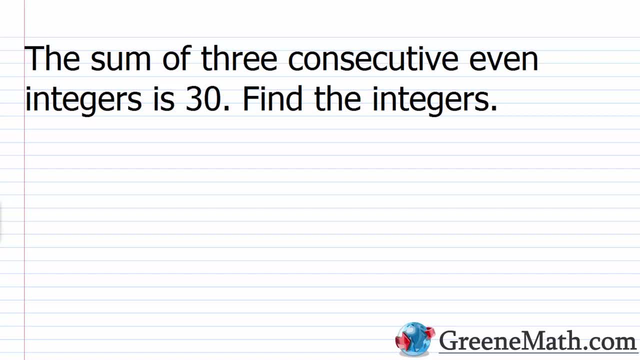 means by saying consecutive even integers. So let's take a look at another one. So the sum of three consecutive even integers. So with that we're talking about again even numbers are numbers that are divisible by two, right? So this is 0,, 2,, 4,, 6,, 8,, 10, 12, things like that. So if I want, 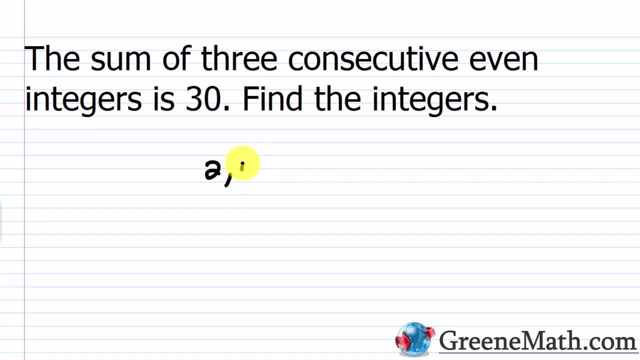 consecutive, even integers. it could be 2,, 4,, 6,, 8,, 10, something like that. It could be starting at 12.. So 12,, 14,, 16,, 18, whatever number you start at, you're just increasing by two each time to get. 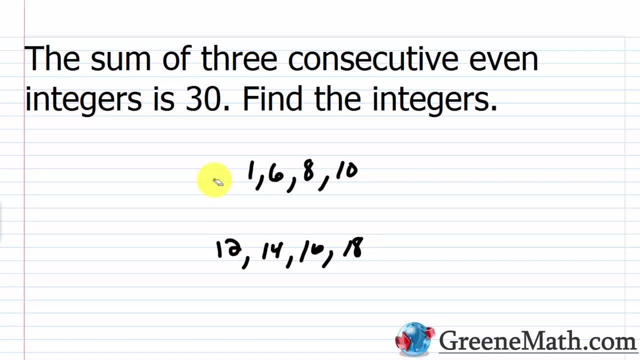 the next even integer. okay, So if I want three consecutive even integers, I can let the smallest just be x. So let x be equal to the smallest even integer. Okay, let me make these e's a little better. So what can we say about the middle one? All right, we have a smallest, we have a middle. 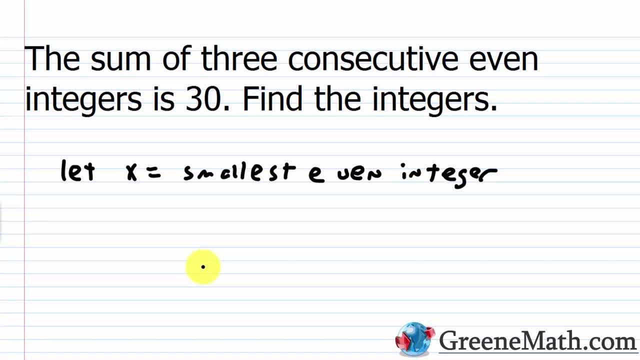 one and we have a largest. Well again, I'm just increasing by two. If I started at two and I went to four, I'm increasing by two. Right, then if I go to six, I'm increasing by two again. So we can say then x plus two is our middle. 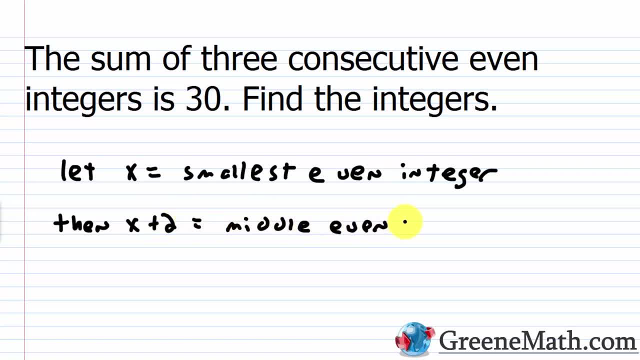 even integer. Okay, let me make that better. And then what We could say then? if I add another two, so x plus two plus another two would be x plus four, So x plus four would be the largest. even So, we're told the sum is 30, right, It's right here. So all we really have to do is take x, which is the. 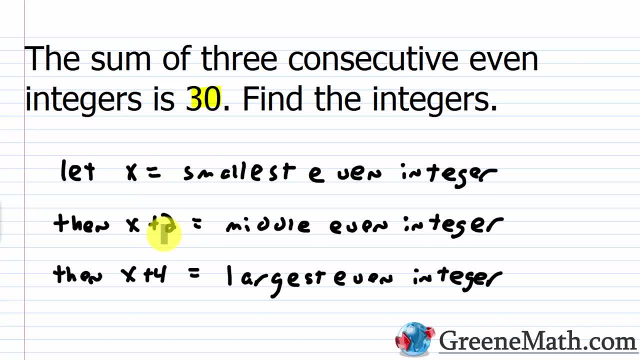 smallest, even integer. add it to x plus two, which is the middle even integer, and add that to x plus four, which is the largest even integer, and set that to 30, solve that equation and we'll be good to go. So we have x plus x plus two plus x plus four. You could wrap these in parentheses, to kind. 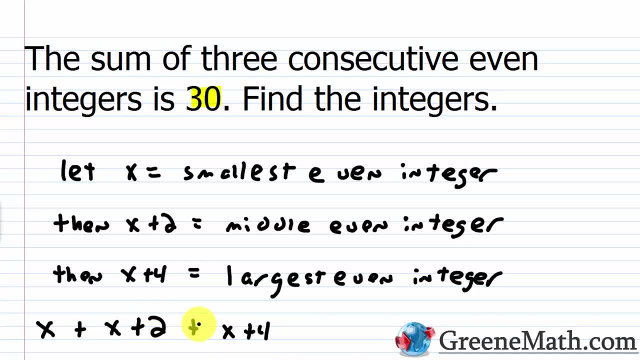 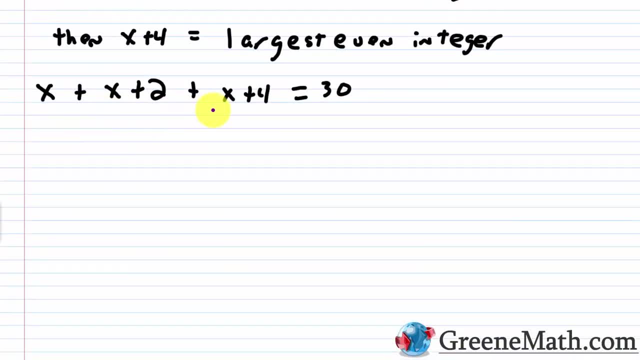 of separate them if you want, but it really serves no purpose, so I'm not going to do that. And this is equal to 30. So let's solve this guy real quick and we'll have our answer. So x plus x plus x is: 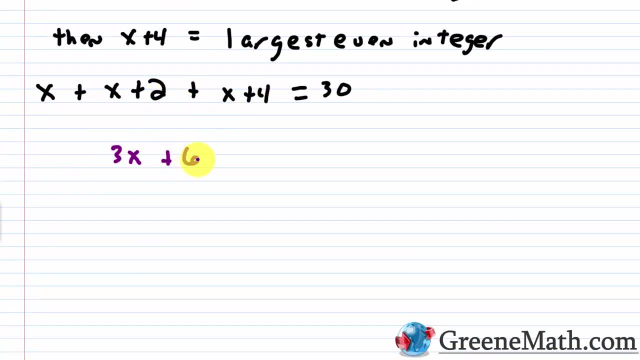 3x, and then two plus four is six. So plus six this equals 30. Let's go ahead and subtract six away from each side of the equation and this is going to cancel. We're going to have: 3x is equal. 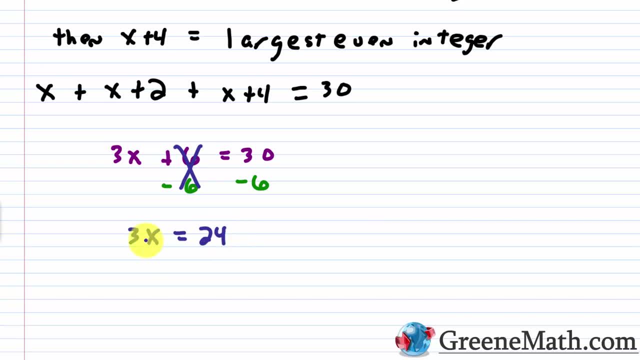 to 30 minus six is 24.. And then I want x by itself. so let's divide both sides of the equation by three. So let's divide both sides of the equation by three. So let's divide both sides of the equation by three and we'll get what This cancels. with this You've got, x is equal to eight. 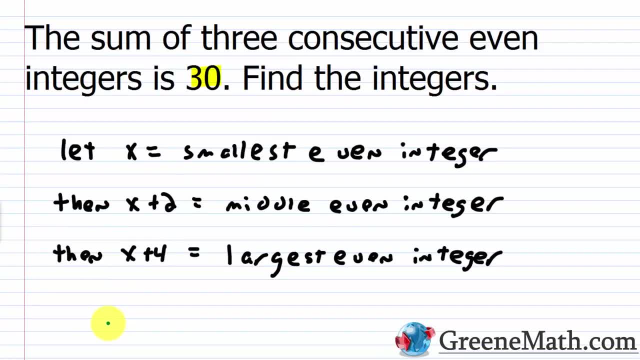 Okay, so let's erase everything Again. the smallest, even integer, was represented with x, so we know that's eight. So then the next even integer would be what? We add two to that, so we get 10, and then add two to that to get to the largest, and that would be 12.. 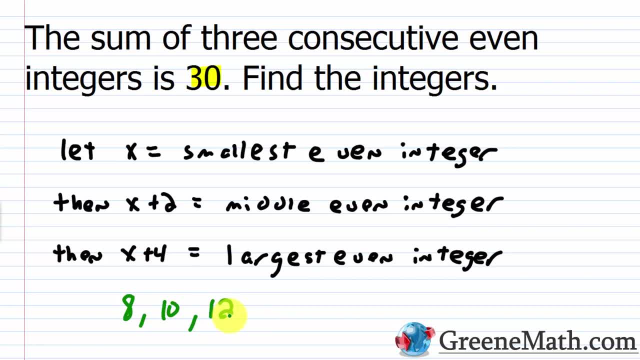 Okay, so the integers would be eight, 10, and 12.. Is that consistent with the problem? Eight plus 10 is 18, and then 18 plus 12 is 30. So we're basically good to go Right, and they're all even numbers and they're in a consecutive sequence. 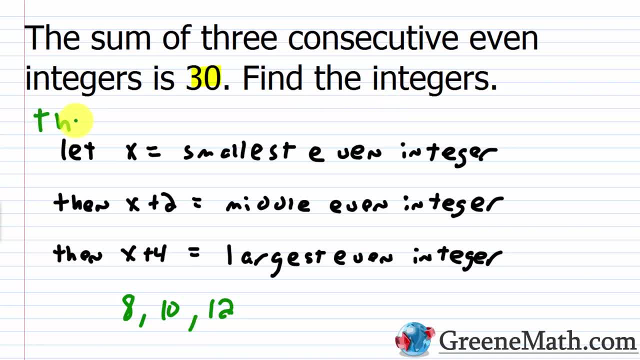 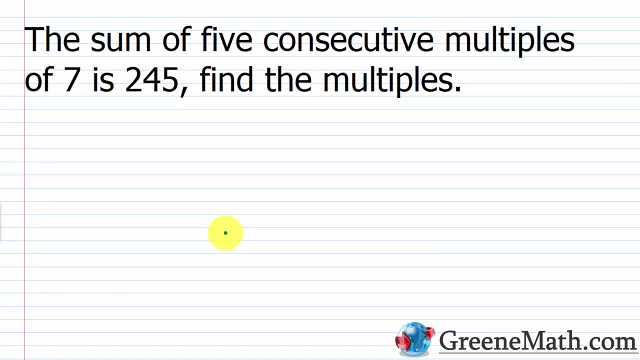 So I can just say: find the integers. The integers are, the integers are, we'll say, eight, 10, and 12.. All right, let's take a look at another one, and this one kind of trips students up, so you just want to pay close attention here. 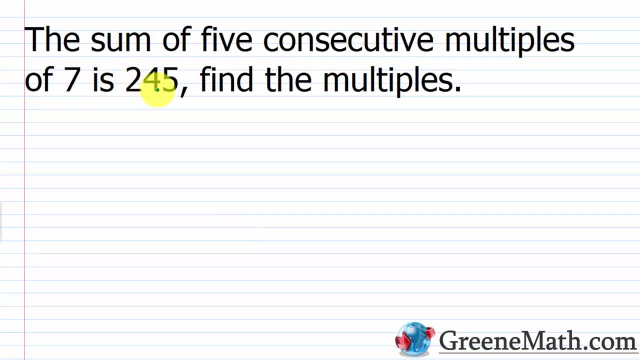 So the sum of five consecutive multiples of seven is 245.. Find the multiple, So the idea here. if you don't remember what a multiple is from pre-algebra, just note that there's multiple definitions of this. but essentially, if I take the number seven, 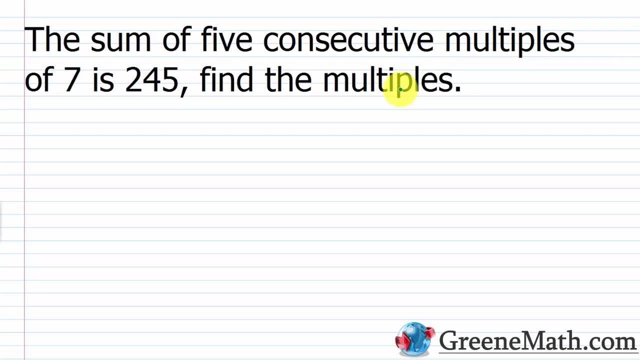 and I multiply it by an integer, so by one or two, or it could be negative seven or whatever. I want to multiply it by. as long as it's an integer, the result there is a multiple of seven. So generally in pre-algebra or a lower-level algebra course you kind of restrict. 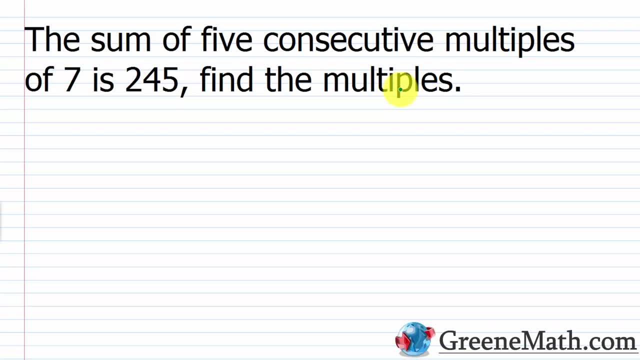 this to: multiplying the number, which in this case is seven, By whole numbers which are one or larger right, So I would say multiples of seven, you'd have seven times one is seven, then seven times two is 14,, then seven times three is 21,. 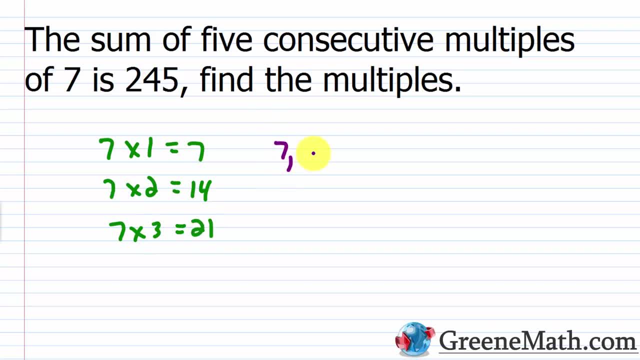 right, So on and so forth. So if I start with seven, then I increase by seven, I get to 14,. increase by seven, I get to 21,. you know so on and so forth. So I go 28,, 35,, 42,, 49,. 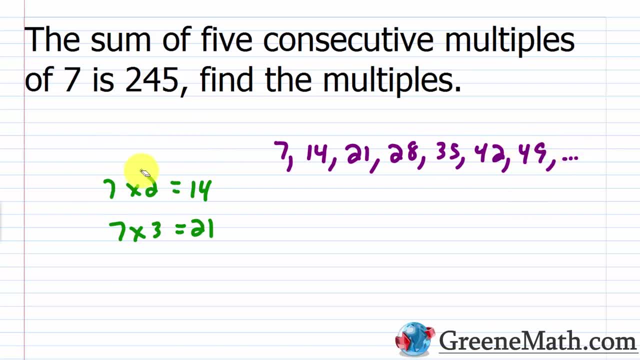 right. This would continue forever. Now, in this particular case, all we know is that we have a multiple of seven, so we have a multiple of seven. need to understand is that each time I go to the next multiple in the sequence, I just add seven. 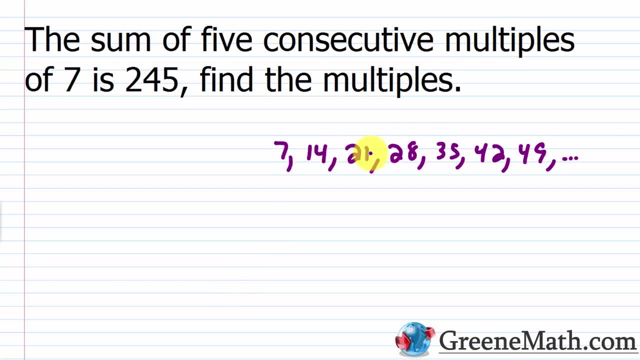 right. So to get from seven to 14,, I add seven. To get from 14 to 21, I add seven. So if the sum of five consecutive multiples of seven is 245, the first multiple could just be x. So let's say: 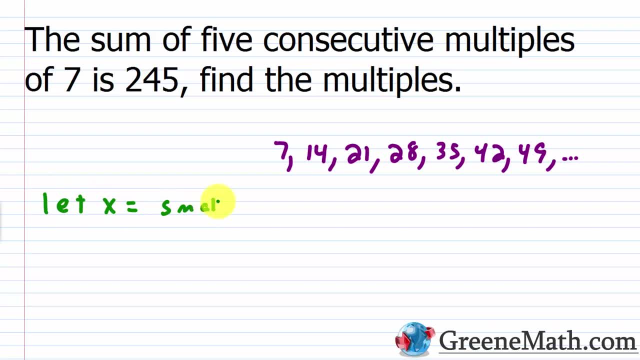 let x be, you say this is the smallest or the first multiple, You'd say, of seven. So then each time I increase to the next multiple I just add seven. So if the sum of five consecutive multiples of seven need to understand is that each time I increase to the next multiple I just add seven. So let's say 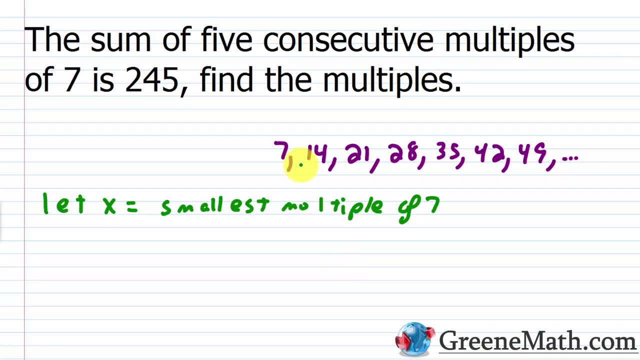 the next multiple. I'm just going to add seven, right, Just to follow this pattern. So we could say then x plus seven is what It's the next number in the sequence, So we would say the next largest, Okay. And then, following this pattern, you're just going to keep adding seven, So we 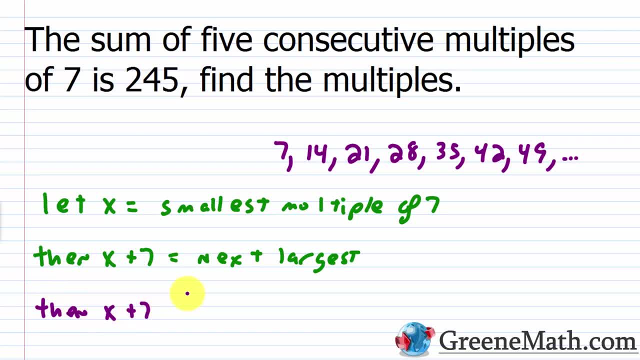 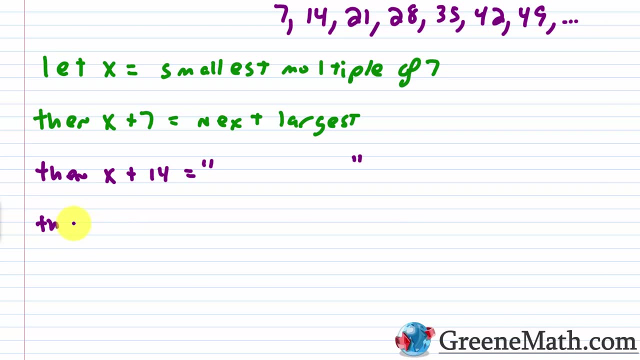 could say: then x plus seven plus seven or x plus 14 would be what, It would be your next largest. So you just keep going until you have five of these guys. So we would say: then let me make that e better, You'd have x plus 14 plus seven, which is x plus 21,. 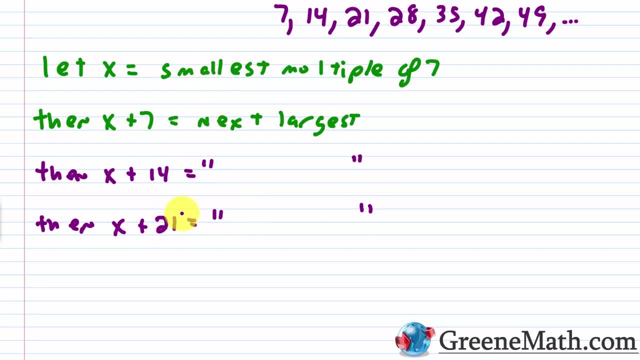 is again the next largest. So you have one, two, three, four. you need one more. So then we could say: x plus 28 is now going to be your largest. Let me write that out. So this would be your largest. 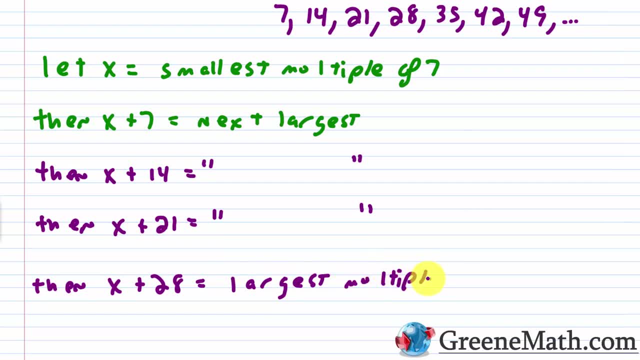 And I'll be specific here and say multiple of seven. Okay, So now what do we want to do? We're told the sum of these guys is 245.. So essentially, what I got to do is just take x plus x plus seven plus x plus 14 plus x plus 21. 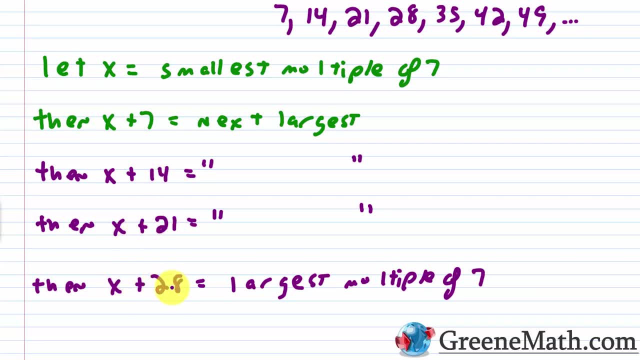 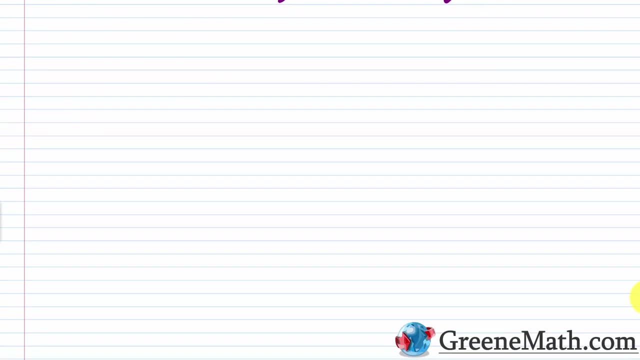 plus x plus 28,. and just set it equal to 245.. Solve that for x and I'll have my answer. Okay, Pretty easy overall. So again I have x plus. the next guy in the sequence is x plus seven plus. the next guy in the sequence is x plus 14. 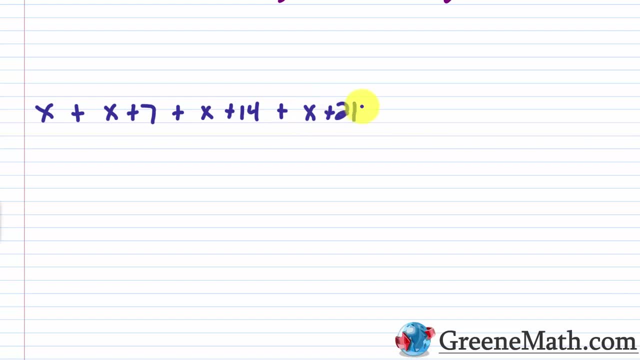 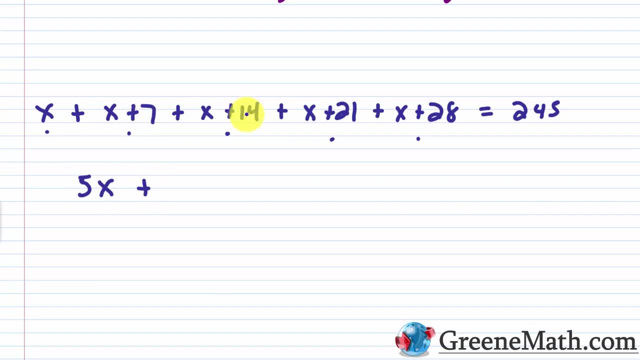 So it's 5x, and then plus, you've got seven plus 14, 21 plus 28, which is 7. okay, so then this equals 245. if i want to solve this for x, i'm going to subtract 70 away from both sides of the equation. so this guy is going to cancel. you'll have 5x. 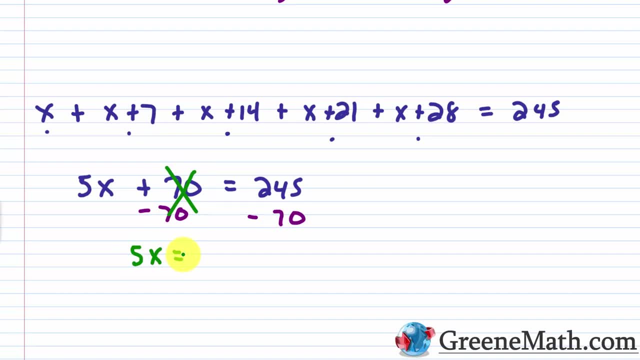 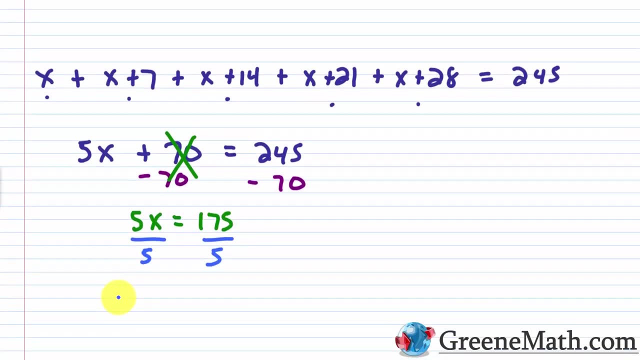 is equal to 245 minus 70 is going to give me 175, and now what we can do is divide both sides of the equation by 5 so we can isolate x and we'll get that x is equal to 175 divided by 5 is 35. 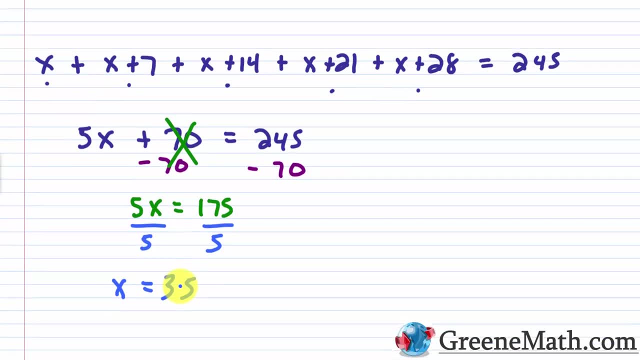 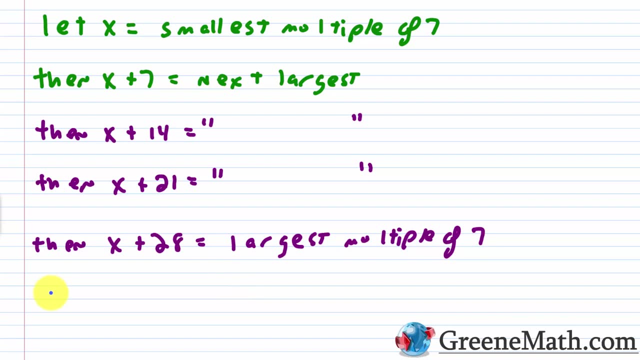 okay, so let's make sense of this. so x is 35. let's go back up. so we said x was the smallest multiple of 7, so the next largest would be plus 7, so we would get 35. add 7, you would get 42. 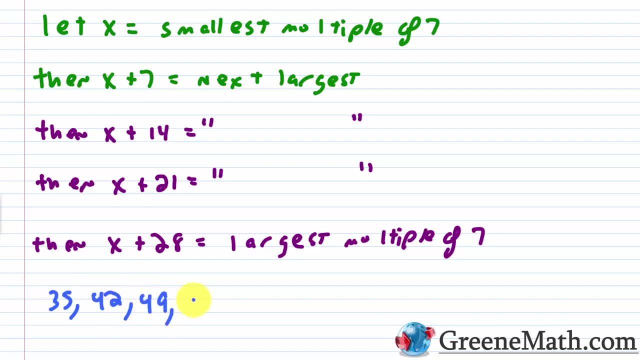 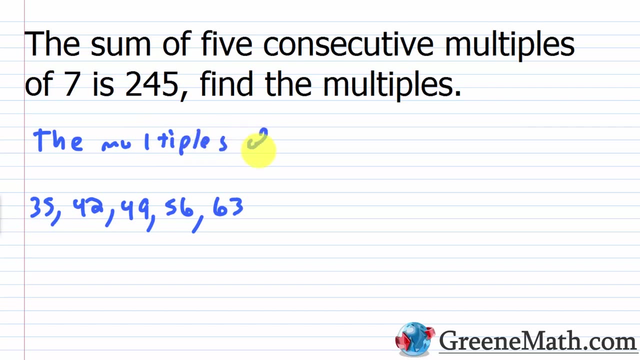 again keep adding 7, so you get to 49, you would get to 56 and then finally you would get to 63. so these are your multiples of 7. so let's erase this, all right. so let's say the multiples of 7 are again: you have 35, 35, 42, 49, 56 and 63. now if you sum these, do you get 245, right, we know? 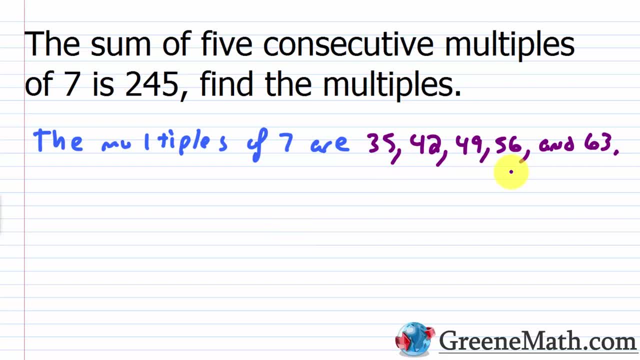 that they're multiples of 7. that's very easy to see. but if we sum these, do we get 245? well, 35 plus 42 is 77. then if i add 49 i get 126, then if i add 56, i get 182, and then finally, if i add 63, i do get 245. so when i sum these numbers, i do get 245. 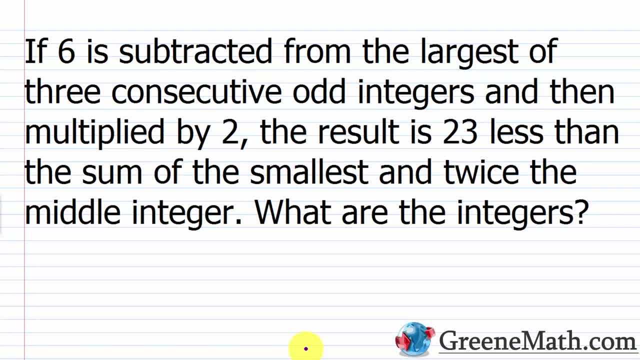 so my solution here is correct. all right, let's take a look at one more problem. so if 6 is subtracted from the largest of three consecutive odd integers and then multiplied by 2, the result is 23 less than the sum of the smallest and twice the middle integer. what are the integers so when? 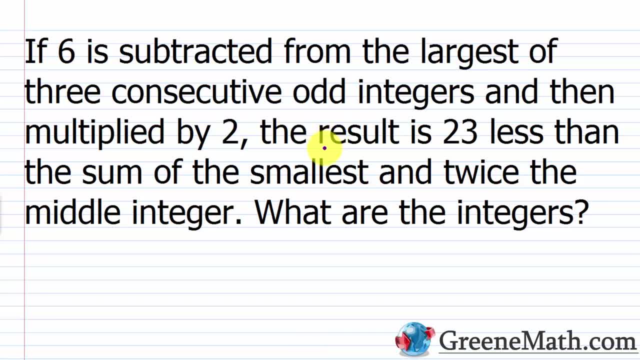 you get a problem like this, you just have to stop and go step by step. okay, if you try to go too fast you might miss a part. this is one of the ones that's just meant to kind of confuse you. so the first thing is it says consecutive odd. 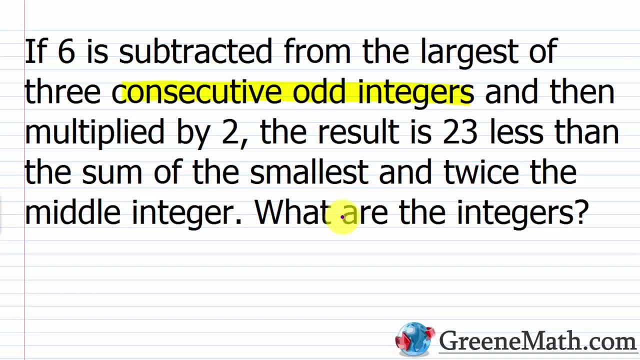 integers. think about the fact that if you have consecutive, even integers, it's 2, 4, 6, 8, 10, right, so on and so forth. odd integers are integers that are not divisible by 2. so if they're consecutive, it's going to differ by 2, so something like 1, 3, 5, 7 and so on and so forth. so if you have consecutive, 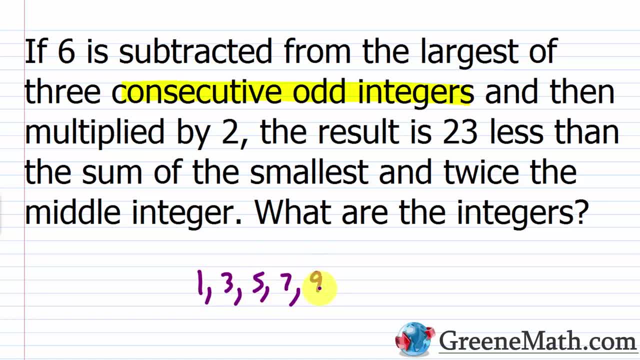 odd integers. it's going to be 1, 4, 6, 7, 9 and just increasing by two once i start with an odd integer. so to kind of model this: let's let x, let's let x be the smallest odd integer, and then we can say that x plus 2 is going to be the middle one. so this is the middle odd integer. i'm going to write this as 3, so i'm going to write length times数 and i'm going to write length times 2, okay, and then the last thing i'm going to do is i'm going to go ahead and do a little bit of something here and i'm going to do this, and then i'm going to go ahead and do this and this is going to go to the next one. so let's write this as the middle odd integer. 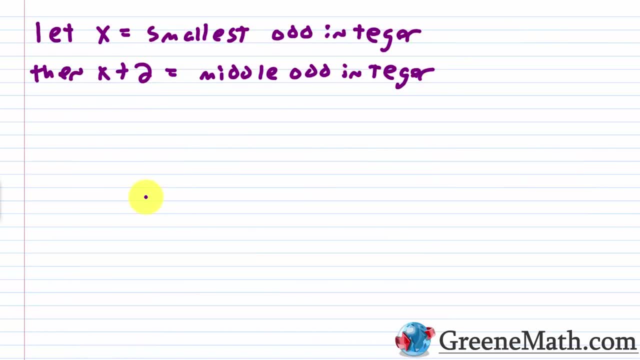 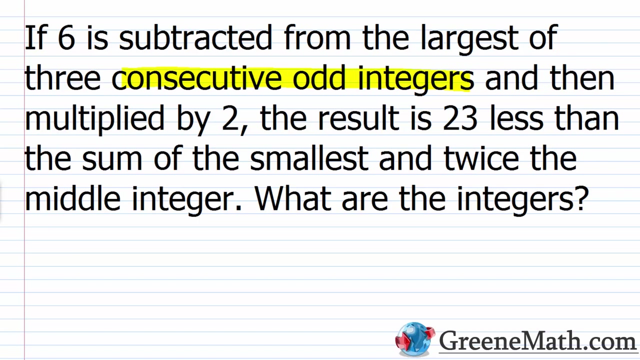 run out of room, so let's take this to another page and so we can also say: then x plus 2 plus 2, which would be x plus 4, is the largest, okay, the largest odd integer, okay. so now that we've modeled the odd integers, that sequence, let's go back up and let's think about what it's saying. if 6 is, 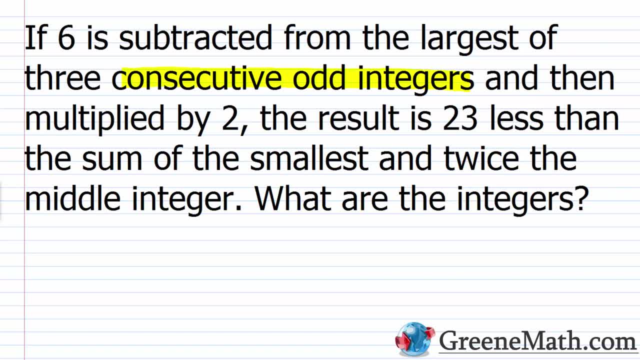 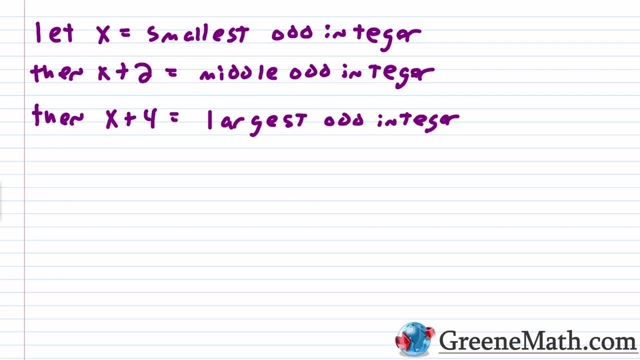 subtracted from the largest of three consecutive odd integers. okay, so 6 is subtracted away from the largest. so the largest we said was x plus 4. so 6 subtracted away, we'd have x plus 4 minus 6, which would translate into x minus 2. okay, so let's just write that. so let's put this as x minus 2. 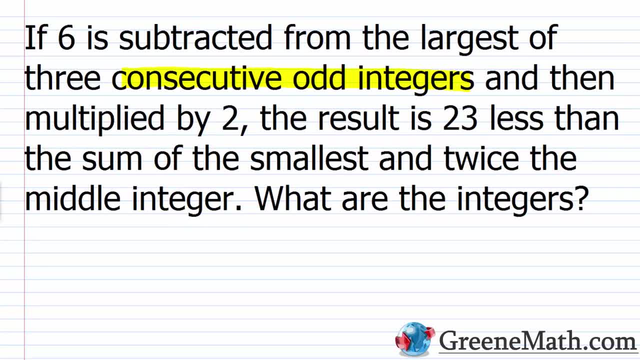 and it says again: if 6 is subtracted away from the largest of three consecutive odd integers, which we've already done, and then okay, so and then. so it's done, after the fact, multiplied by 2. so we're going to multiply this guy by 2. this is a quantity. x minus 2 is a quantity. 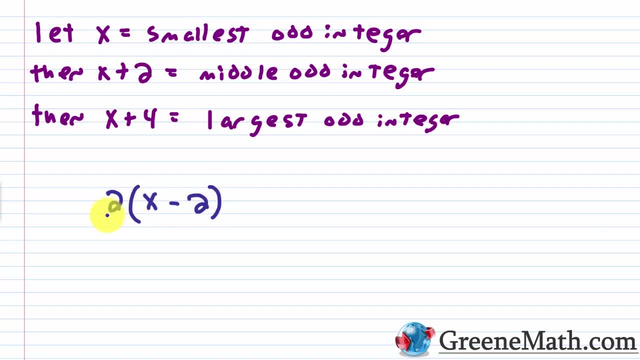 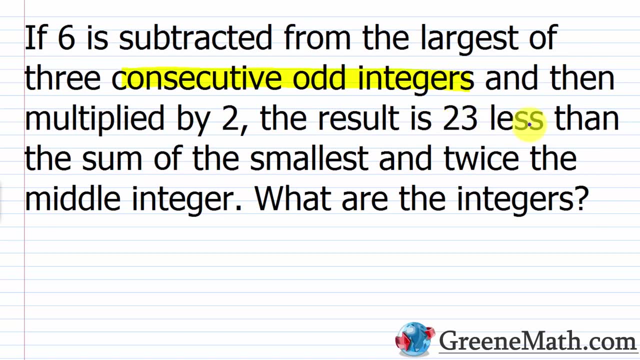 so i've got to multiply the quantity x minus 2 by 2. then it says the result is: so that always means equals. so again, the result is you have 23 less than the sum of the smallest and twice the middle integer. okay, so this is a lot to unpack. so we know that we're subtracting 23 away from. 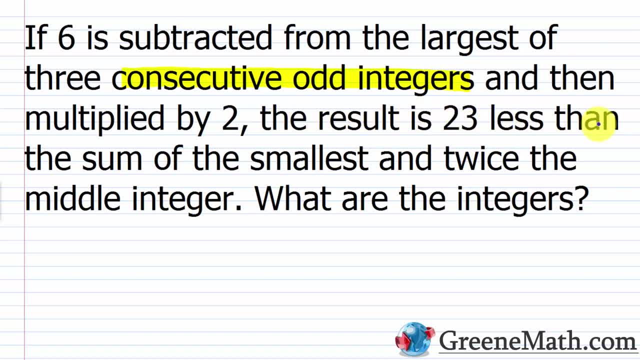 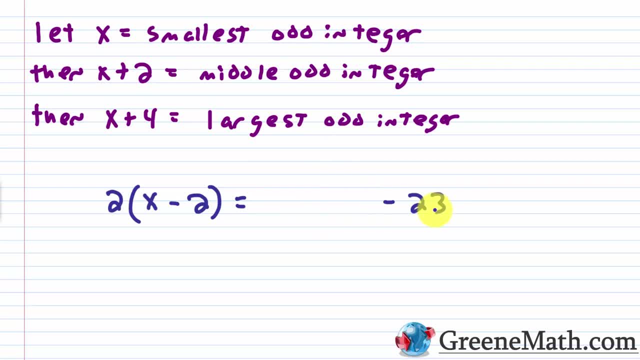 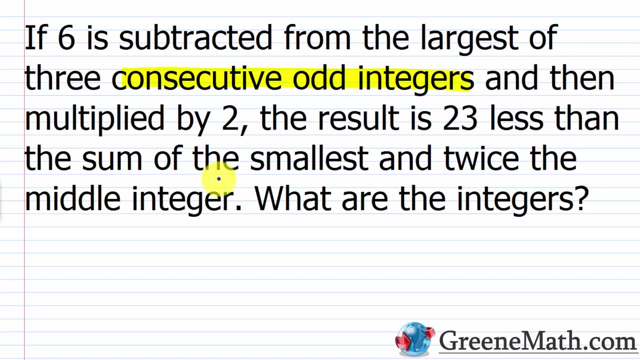 something, because it says the result is 23 less than so. let's go back here. i'm just going to put minus 23 out here because we're going to do something, and then we're going to subtract 23 away. now it says the sum of the smallest, which we said was x, and twice the middle integer. 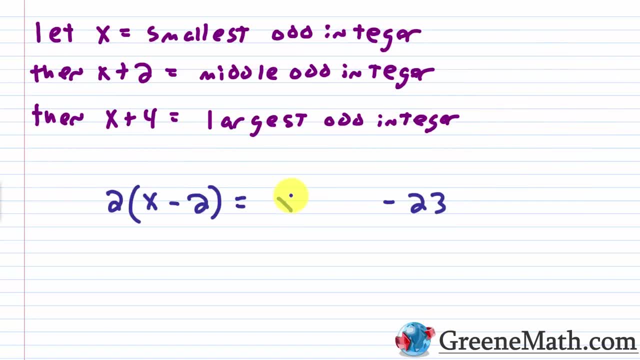 the smallest, which we said was x and twice the middle integer. we want that sum. the middle integer is x plus 2. so again i've got to use some parentheses here, so let me kind of drag this over. so 2 times this quantity, x plus 2, okay, so let's read through this: 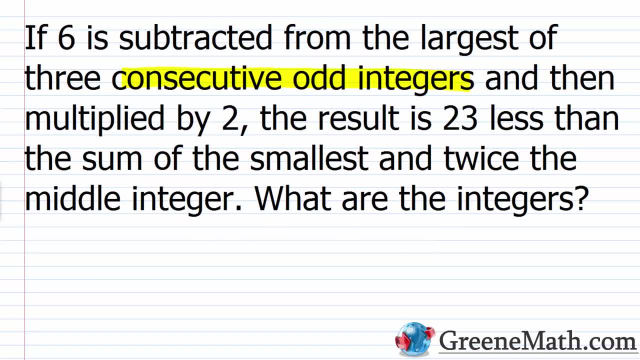 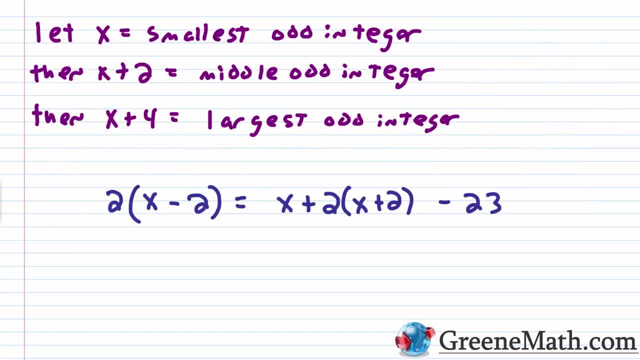 again and make sure we understand where this came from. so again, if 6 is subtracted from the largest of three consecutive odd integers and then multiplied by 2- so essentially we started with the x plus 4 is the largest odd integer. we subtracted away 6. that's how we got x minus 2. 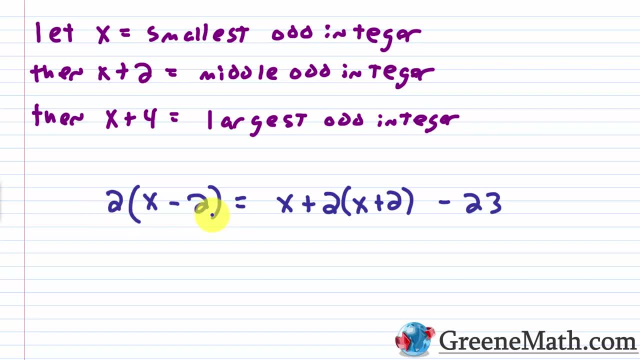 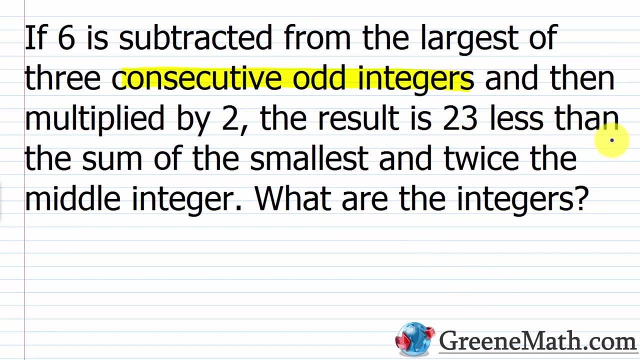 and then we multiplied by 2 to get the left side. then it tells us the result is: so. that's where we got our equal sign from. if you say the result is, you're basically saying is equal to. so on the right side we have that it's 23 less than the. 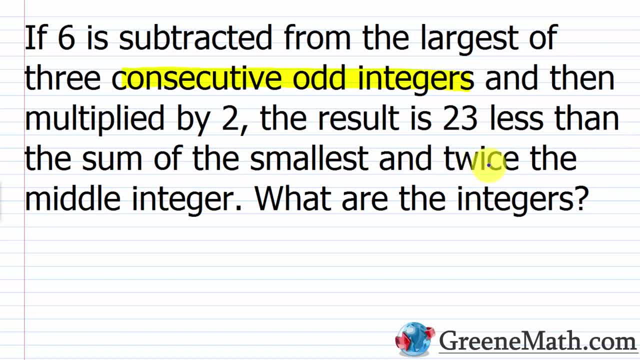 sum of the smallest, which are represented with x, and twice the middle integer. now the middle integer is x plus 2, so twice the middle integer is 2 times the quantity x plus 2. so that's where you got this from. the sum of the smallest integer and then multiplied by 2. so that's where you got this from. 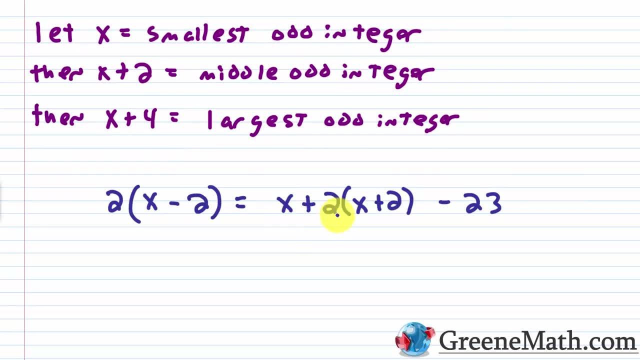 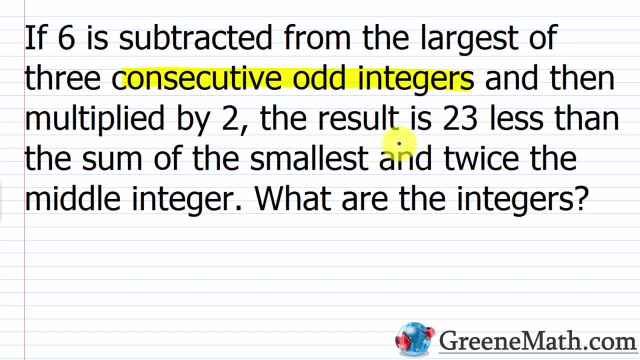 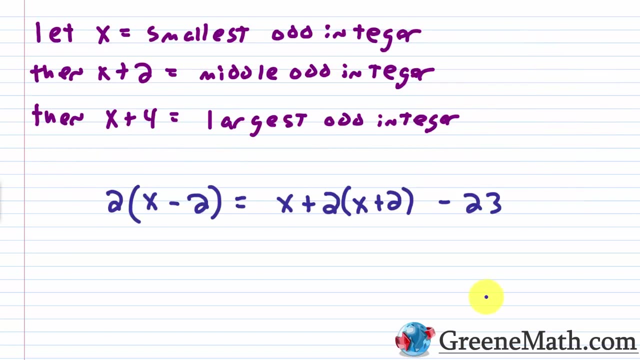 which is x, and twice the middle integer, which is 2 times x plus 2. so we sum those two together and then we need to subtract 23 away from that, because it says the result is 23 less than okay. so now that we have this set up again, these are kind of a pain to get to this point. 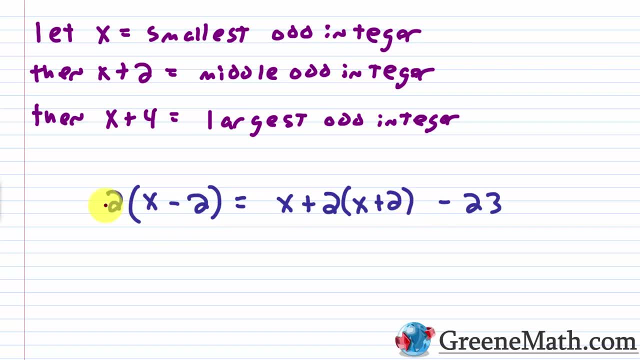 but once you have it, it's pretty easy. you're solving an equation. so clean up on the left: 2 times x is 2x, then minus 2 times 2 is 4. this equals you have x plus 2 times x is 2x, and then plus 2 times 2 is 4, and then minus 23. okay, so let's think about this on. 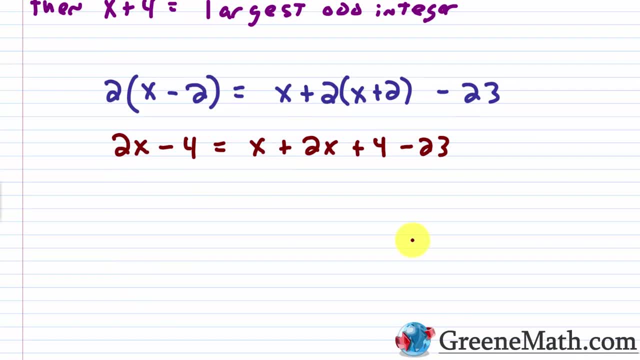 the left side nothing i can do on the right side. i can take x and add to 2x. that would give me 3x, and then 4 minus 23 is negative 19. again over here i'm just going to write 2x minus 4, nothing's. 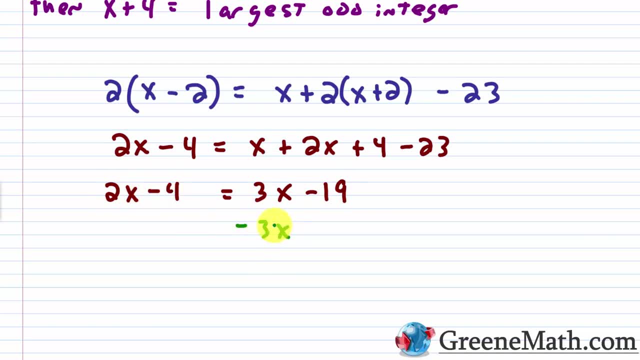 going to change. i'm going to subtract 3x away from each side of the equation and i'm going to add 4 equation. So what's going to happen is this guy right here is going to cancel and this guy is going to cancel. 2x minus 3x is negative x and this equals negative 19 plus 4 is going to be. 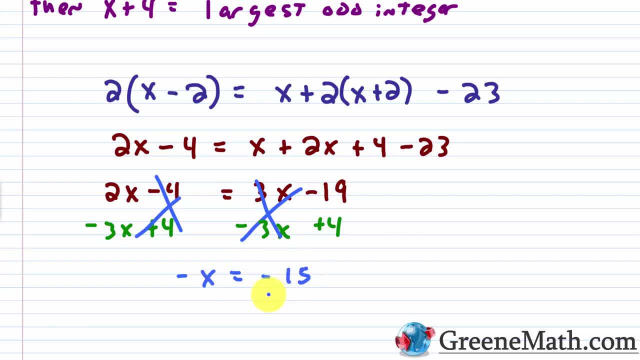 negative 15.. Now to get x by itself, I can multiply both sides by negative 1 or divide both sides by negative 1.. Makes no difference, You're going to get that x is equal to 15.. Okay, so let's erase. 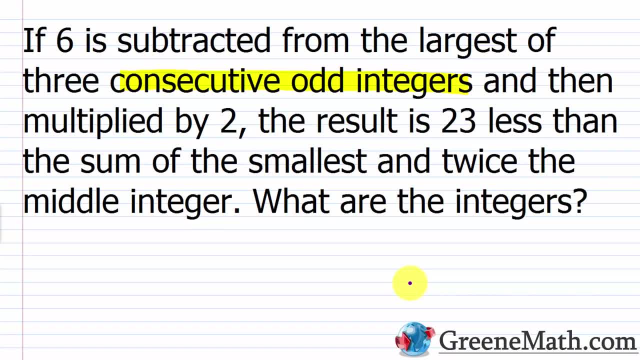 all this. So remember, x was the smallest odd integer. So if we go back up, what are the integers? We'll say the integers are- let me make the e better. So we have 15.. The next one would be 17,. right, if it's consecutive odd integers, And then the last one would be 19.. Let me put. 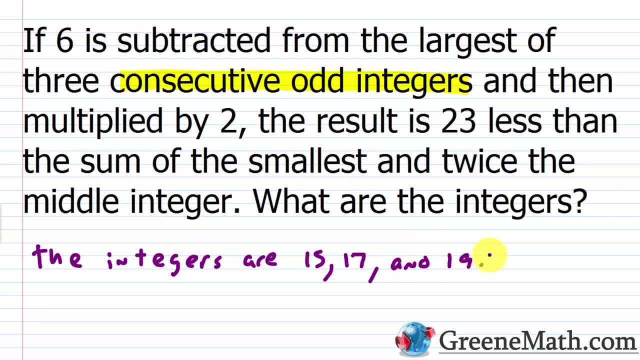 and 19 here, So and 19.. Okay, does this make mathematical sense? Normally with these problems you just get a straight sum, so it's very easy to check, But this one you have to do a little bit of work. So if 6 is subtracted from the largest of three consecutive odd integers, 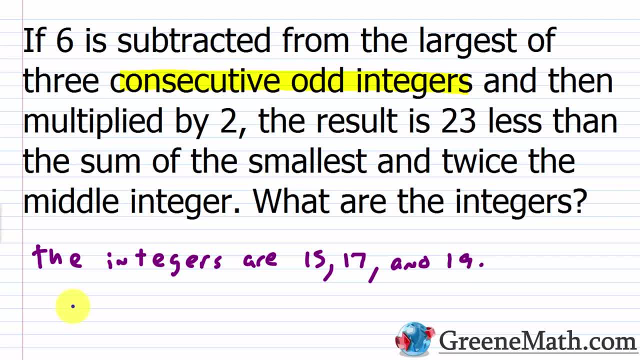 so the largest is 19.. If I take 6 away, I'd have 13.. Then it tells us: and then multiply it by 2.. So 13 multiplied by 2 is 26.. So this is 26. And it says the result is: so this is equal to. 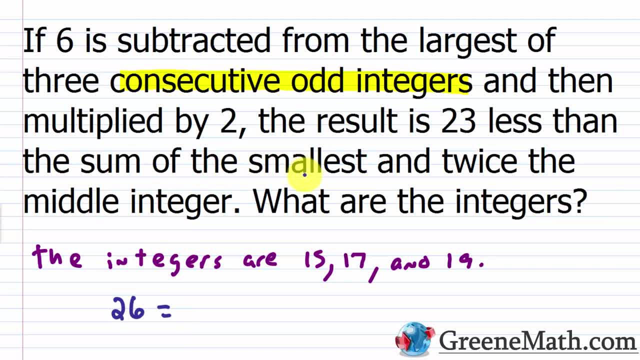 so we have 23 less than the sum of the smallest. So the smallest is what? It's 15. Plus twice the middle integer, The middle integer is 17.. So if I take 2 and multiply it by 17,, I get 34.. And again, it's 23 less than this. So I'm going to subtract 23 away from this.